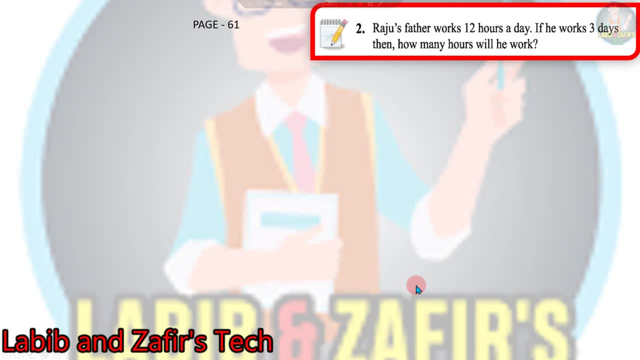 So, students, I have done some word problems about 10 word problems in my last video, So today I am again going to show some another 10 word problems, So let's start. So at first we have a word problem from page 61, part 2.. Raju's father works 12 hours a day. If he works 3 days, then how many hours will he work? 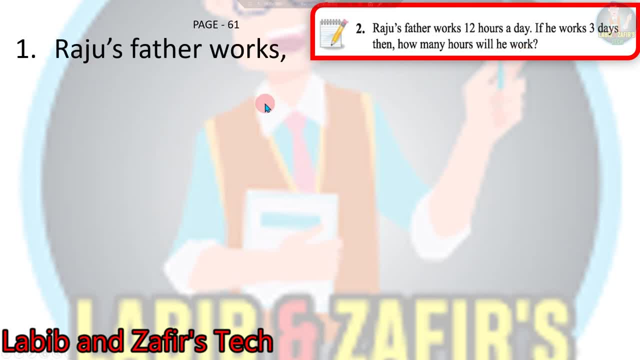 So, students, at first, Raju's father works in 1 day 12 hours. So in 3 days 12 into 3 hours. so that is is equal to 36 hours. So here, if we multiply 12 by 3, 3 into 2 is equal to 6, and 3 into 1 is equal to 3.. That is 36 hours. So Raju's father will work 36 hours in 3 days. 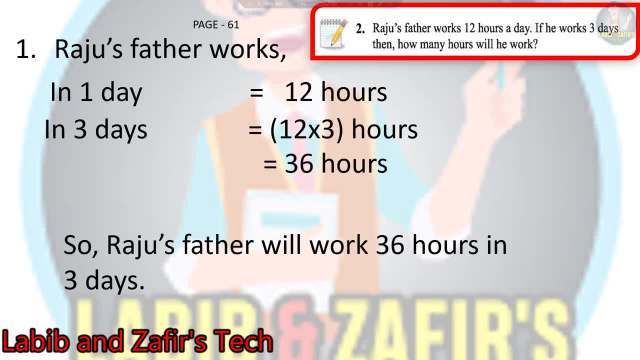 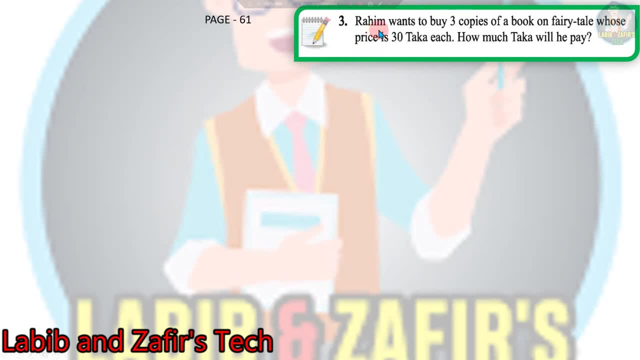 So, students, this is the first word problem. Now I am going to show you the next one. So there, students, this is the next word problem from page 61 again, Rohim wants to buy 3 copies of a book on fairy tale whose price is 30 taka each. How much taka will he pay? 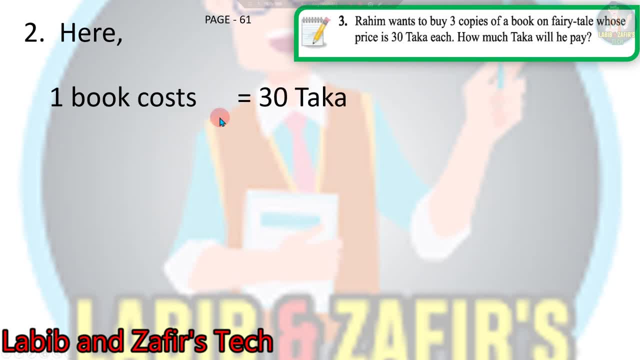 So students, at first number 2 here: 1 book cost 30 taka. 3 book cost 30 into 3 taka. That is, if we multiply 30 into 3, that will be 90. here 3 into 0 is equal to 0 and 3 into 3 is equal to 9.. That is 90 taka. 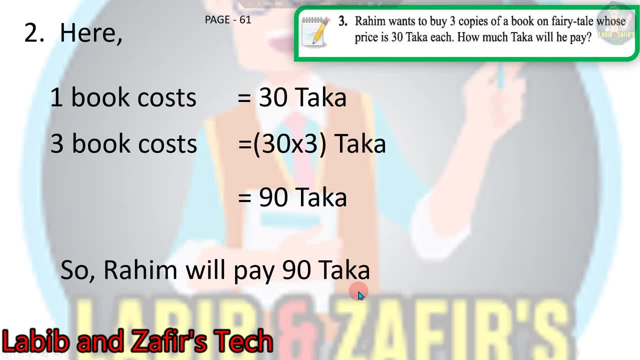 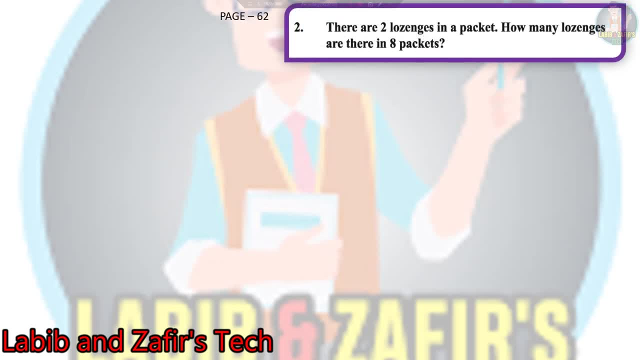 So Rohim will pay 90 taka. So these are the word problems from page 61.. Now I am going to show you the another word problem. So, students, now we are in page 62. It is our third word problem. 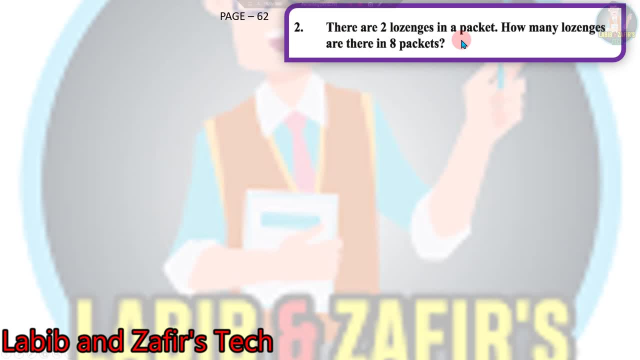 There are 2 logins in a packet. There are 2 logins in a packet. There are 2 logins in a packet. How many logins are there in 8 packets? So students at first we can see here: in 1 packet there are 2 logins. 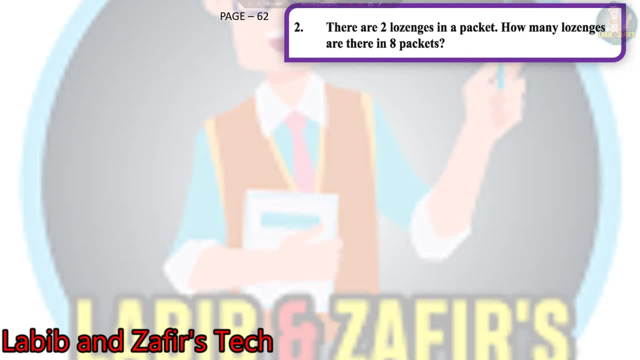 So we have to find the number of logins in 8 packets. So, students, now I am going to show you the solution. But 3 given In 1 packet. there are 2 logins In 8 packets. there are 2 into 8 logins. 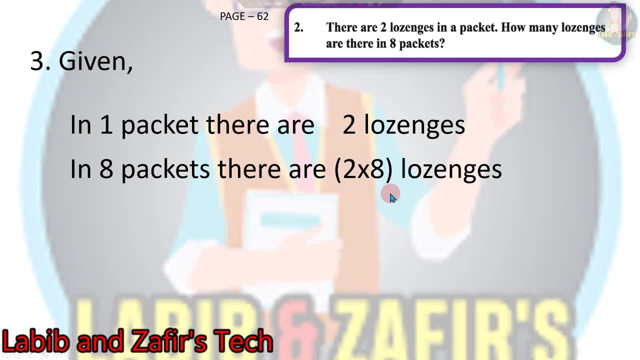 That is, if we multiply 2 into 8, that will be 16 logins. So that is so: there are 16 logins in 8 packets. So, students, this is the third word problem with solution. Now I am going to show you the next one. 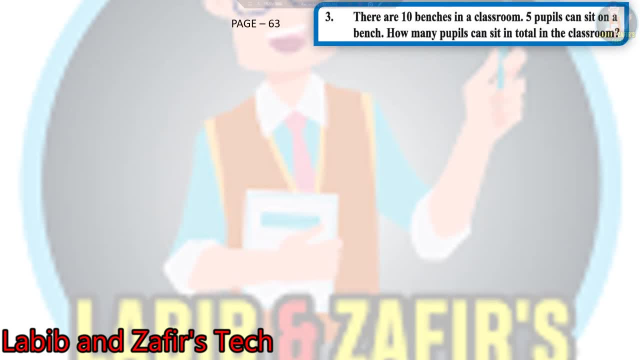 So, students, this is from page 63.. So here we can see. there are 10 benches in a classroom. 5 pupils can sit on a bench. How many pupils can sit in total in the classroom? So, students, for your understanding, I am going to describe what is pupils. 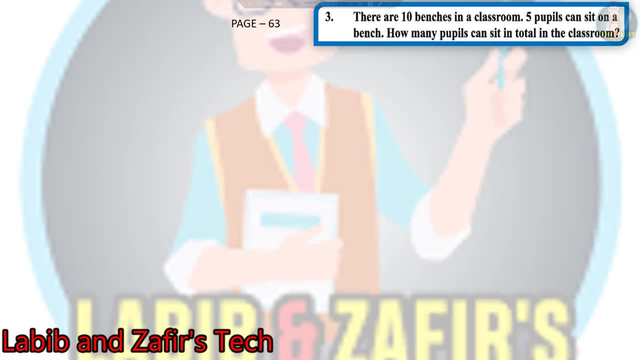 Pupils is the synonym of students. So here we can see pupils and students are the same meaning. There is the same meaning. So at first we can see here in 1 bench there are 5 pupils can sit. So how many pupils can sit in 10 benches or in the total classroom? 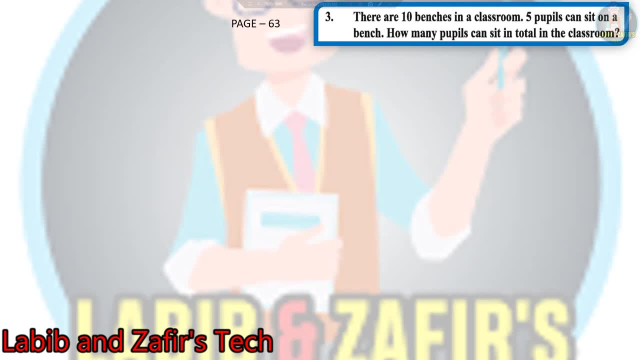 As you can see, in the total classroom there are only 10 benches. So now I am going to show you the solution number 4 here. In 1 bench can sit 5 pupils. In 10 benches can sit 5 into 10.. 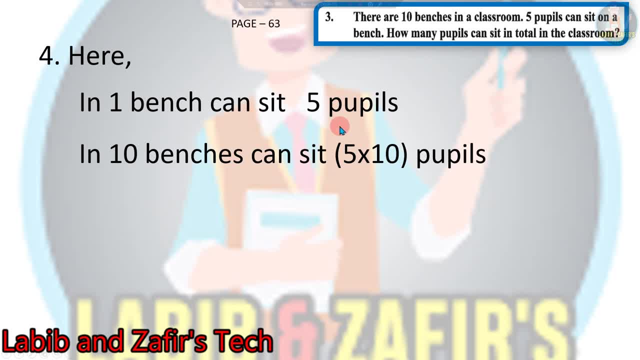 As you can see here, in 1 bench can sit 5 pupils can sit. So we have to find the number of pupils in 10 benches. So we have to multiply 5 by 10. So that is 50. So here 5 into 0 is equal to 0.. 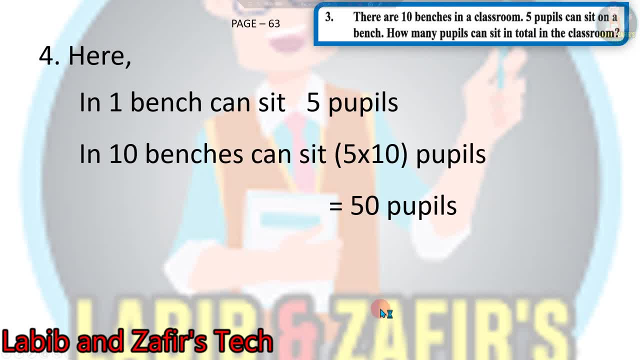 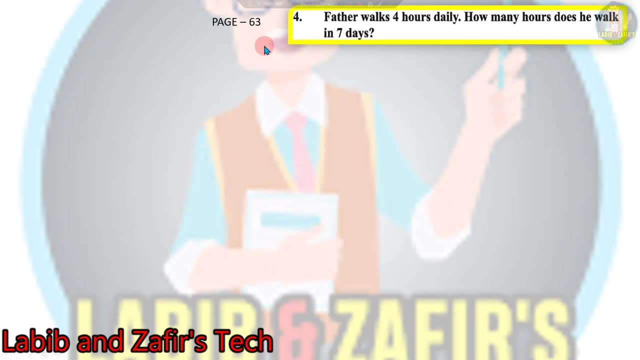 5 into 1 is equal to 5. That is 50 pupils. So 50 pupils can sit in total in the classroom. So this is the fourth question. Now I am going to show you the fifth one. So again from page 63.. 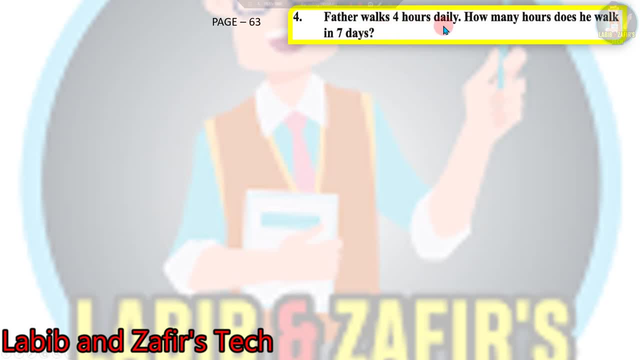 Father works 4 hours daily. How many hours does he work in 7 days? So does he work in 7 days? So, students, we can see in 1 day. father works 4 hours, So we have to find how many hours does he work in 7 days. 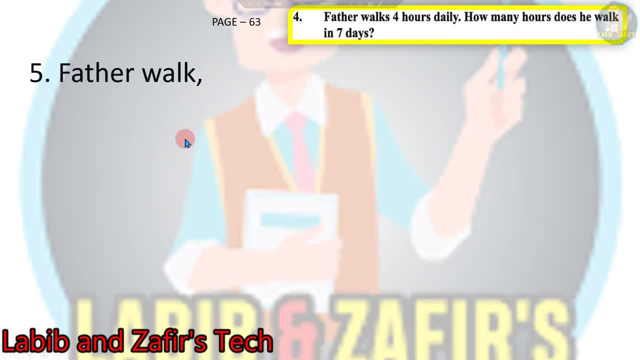 So now we will see the solution. Father works in 1 day 4 hours, So in 7 days 4 into 7.. Here we can see: in 1 day he works 4 hours, So we have to find how many hours does he work in 7 days? 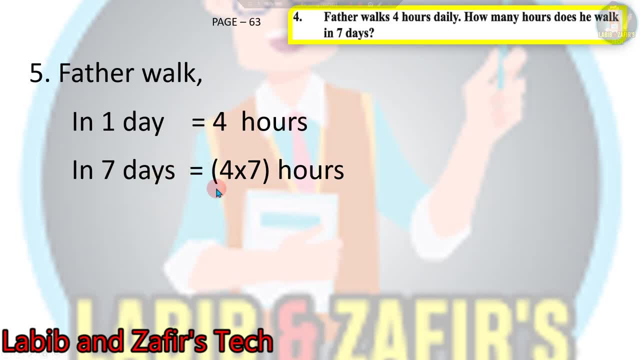 So we have to multiply this 4 by 7. That is, 4 into 7 is equal to 28 hours. So father will work 28 hours in 7 days. Now, students. now I am going to show you the next question. 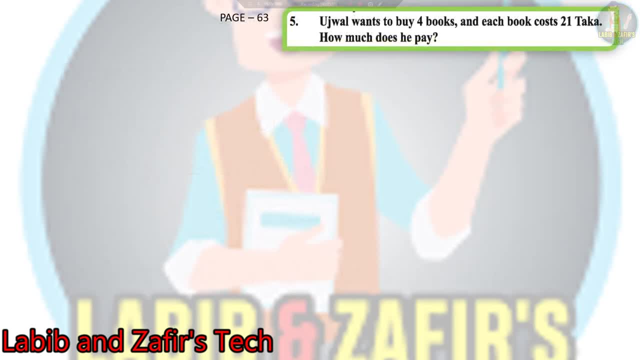 So this is again from page 63.. Ujjal wants to buy 4 books and each book costs 21 taka. How much does he pay? So, students, at first we can see: Ujjal wants to buy 4 books and each of the books costs 21 taka. 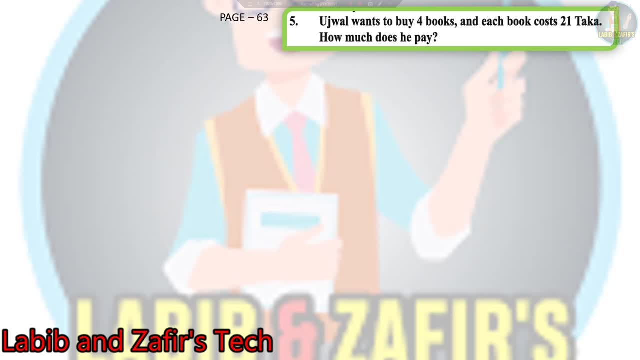 So, students, we can see 1 book costs 21 taka. So we have to find how many taka does 4 books cost? Then that will be the answer, that how much money will Ujjal pay? Now we will see the solution. 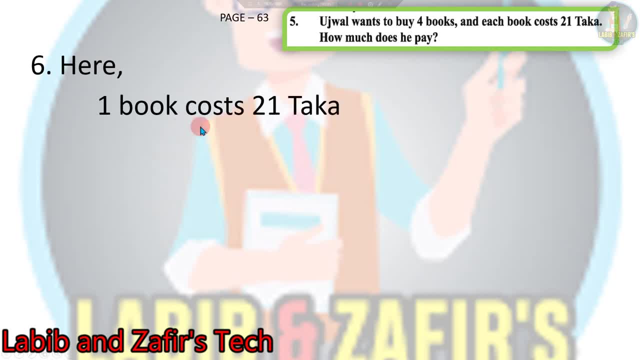 So number 6 here. 1 book costs 21 taka. 4 books cost 21 into 4.. As you can see, 1 book cost 21.. So we have to find the cost of 4 books. So we have to multiply 21 by 4.. 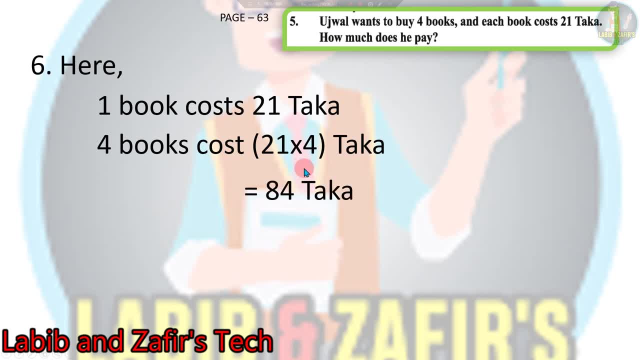 That is, 21 into 4 is equal to 84. Here 4 into 1 is equal to 4. And 4 into 2 is equal to 8. That is 84 taka. So Ujjal will pay 84 taka. 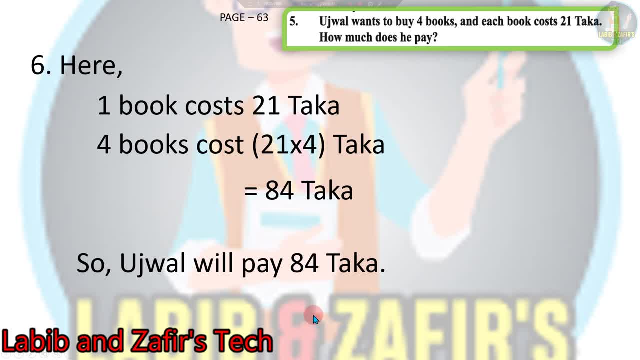 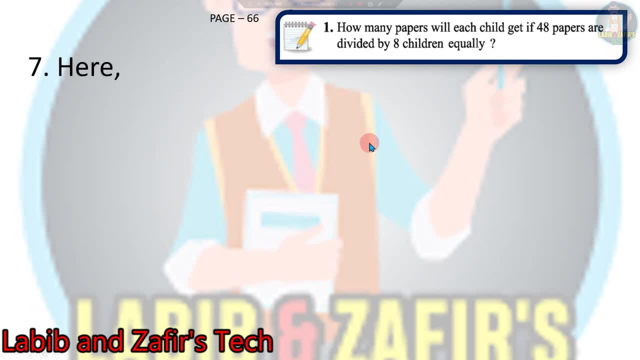 Now next quick word problem. This is from page 66. We are now in another page. So, students here, How many papers will each child get if 48 papers are divided by 8 children equally? So, students, now you can see that now we are in a. this is one kind of divisional word problem. 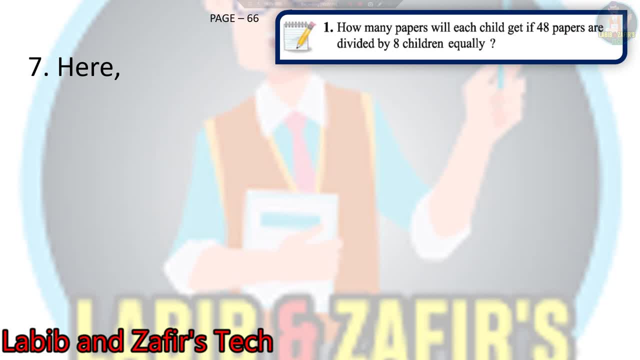 So here it is given that 8 children will get 48 papers. So we have to find how many papers will 1 children will get. So this is a divisional word problem. So number 7: here 8 children will get 48 papers. 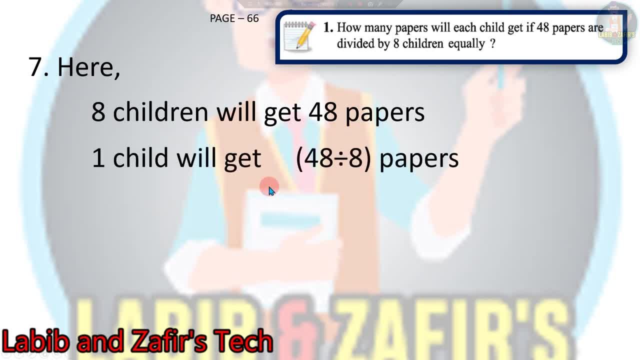 So 1 child will get 48 divided by 8.. So, students, let me make you understand Here: 48 papers will be given to 8 children, So we have to find how many papers will 1 child will get. So we have to divide this 48 papers by 1 child. 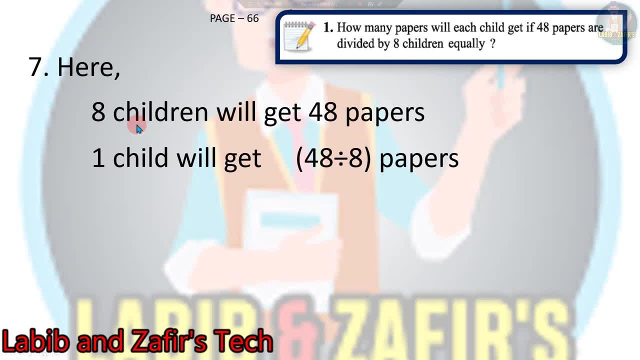 That is 48 divided by 8 children. So 48 divided by 8 is equal to 6.. That is 6 papers. So each children will get 6 papers. Now I am going to show you another word problem. So, students, now we are going to show you another word problem from page 66.. 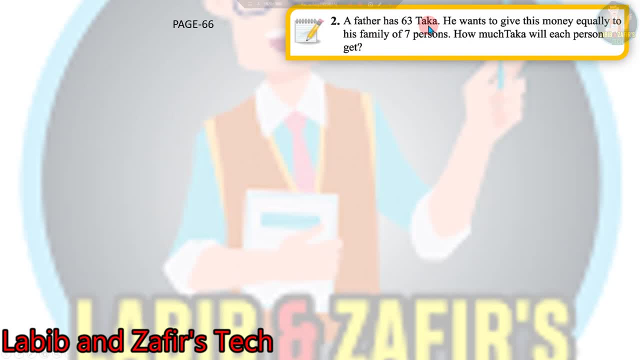 That is, a father has 63 taka. He wants to give his money, To give his money equally to his family of 7 persons. How much taka will each person get? So, students, you can see here: a father has 63 taka. 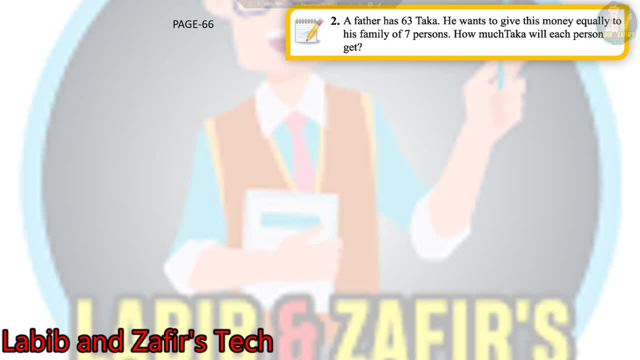 So he will divide this taka into 7 persons of his family. So, as you can see this 7 persons will get 63 taka totally, But we have to find 1 person will get how much taka. So, students, let me see give you the answer. 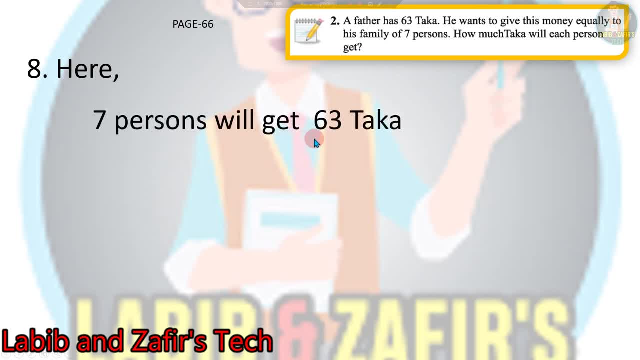 8 here. 7 persons will get 63 taka, So you have to find 1 person will get 63 divided by 7.. As you can see, 7 person will get 63 taka, So 63 will be divided by 7.. 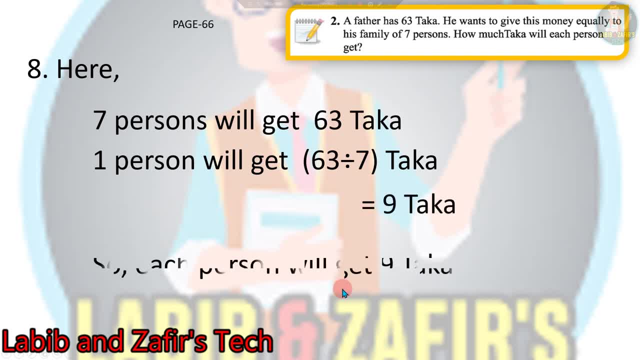 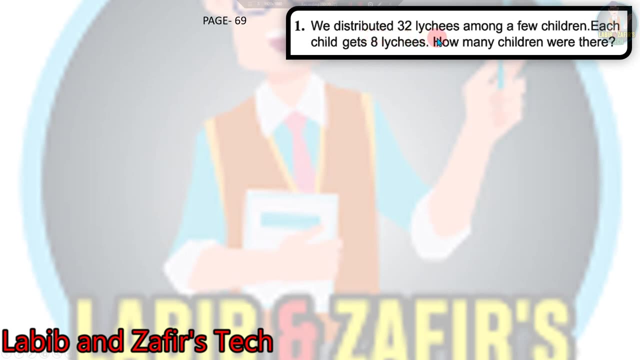 So that is 9 taka. So each person will get 9 taka. Now I am going to show you the 9th word problem. So This is another word problem. We distributed 32 liches among a few children. 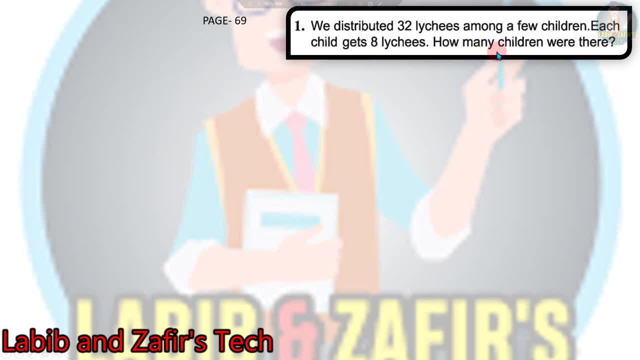 Each child gets 8 liches. How many children were there So, students? this is one kind of critical question, But my solution will make you understand very easily, So let me give you the solution here. So, given, 8 liches were given to 1 child. 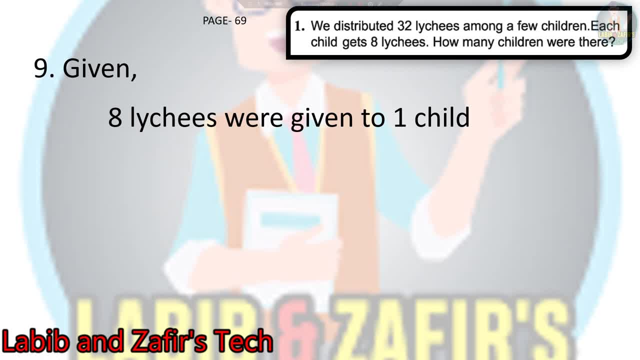 So at first I need to describe that In our last some word problems we have seen that Every, for example, 8 persons got 32 liches or something. So now we have to find how many persons or how many children were there. 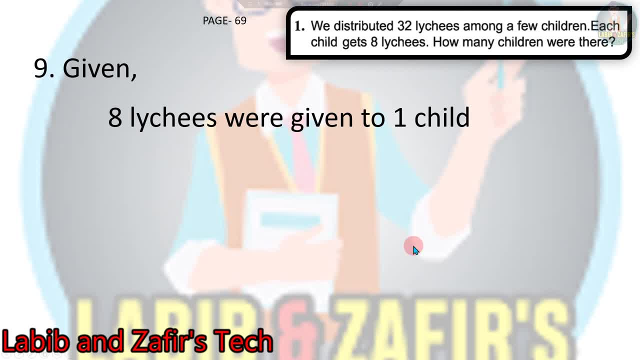 So we can see, 8 liches were given to 1 child. So 32 liches were given to Here. as we can see, 32 liches were given to. We have to find how many children were there And, as we can see, 8 liches were given to 1 child. 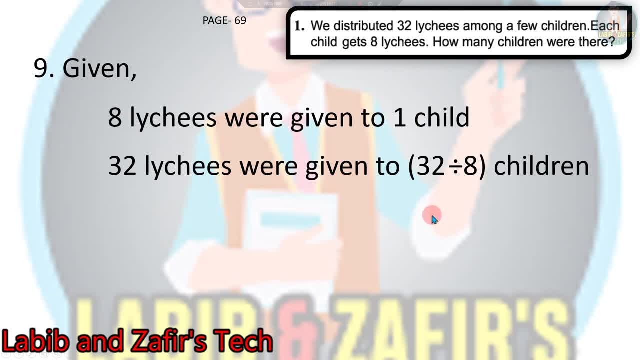 So here we have to divide this 32 by 8. That is 4 children. If you want to prove that this division is right or not, You can multiply this 4 by 8. then you can get this answer: That is 32.. 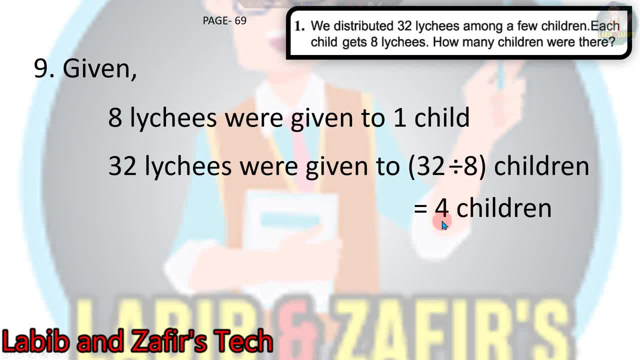 So we can see, 4 into 8 is equal to 32.. And, as we can see, 32 liches were given to 4 children. So there are 4 children. So, students, now I am going to show you the last question for today's video. 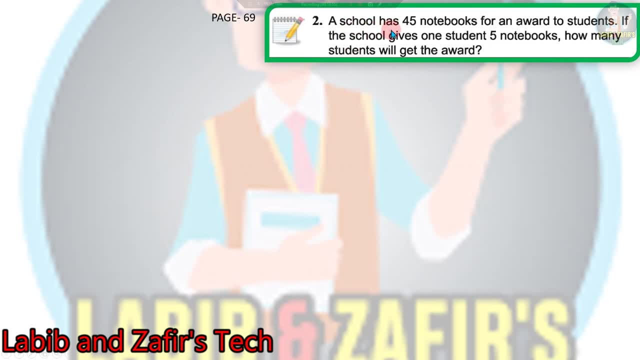 That is. this is the last question. A school has 45 notebooks for an award to students. If the school gives 1 student 5 notebooks, How many students will get the award? So students? this is again the same question, like the last one. 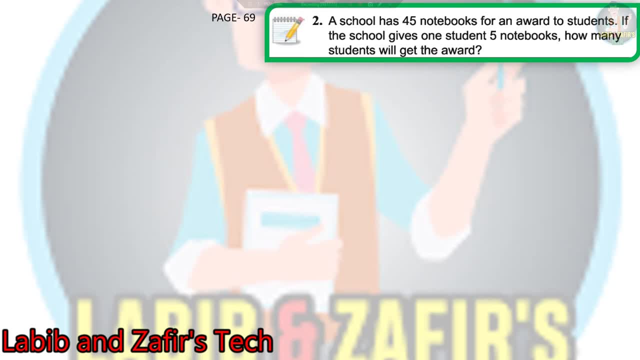 So we have to find How many students were there And, as you can see, 1 information is given there. There are, and each student gets 5 notebooks. So now I am going to show you the solution. So 10 given, 5 notebooks were given to 1 student. 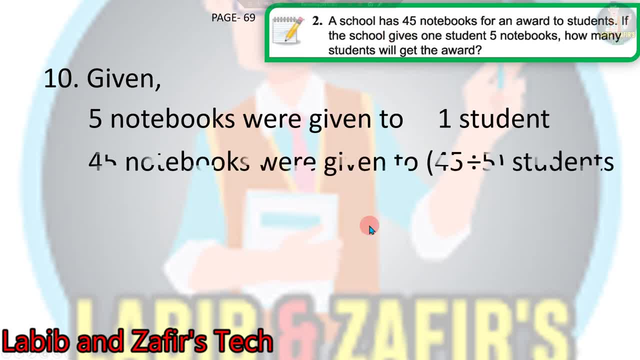 So it is given already in the question. Now we have to find 45 notebooks were given to. Again here we have to divide this 45 by 5. So as we, because we have to know the Number of students who will get the award.